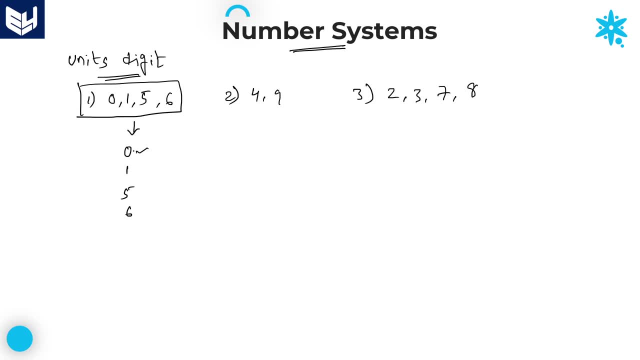 Then its units place is always the same digit. If a number is ending with 0 units, place is 0. Ending with 1 units, place is 1.. Ending with 5 units, place is 5.. Ending with 6 units: place is 6.. Irrespective of the value of power, whatever the power value, whatever the natural number in the power value, your answer will be always the same digit in which that particular number ends. 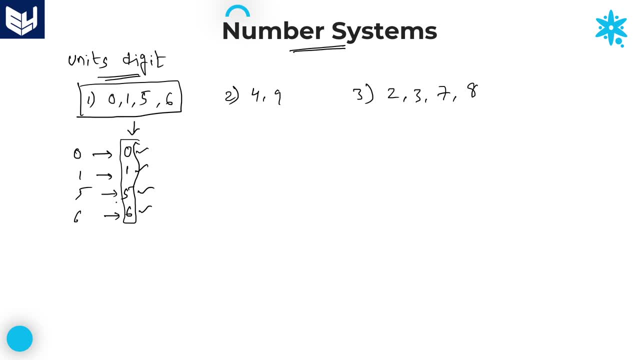 If it ends with 0,, 0,, 1,, 1,, 5,, 5,, 6,, 6.. Related to units: place digit. In the last session I explained only the concept. Now, in this session, I will explain the examples of this particular first category digits. 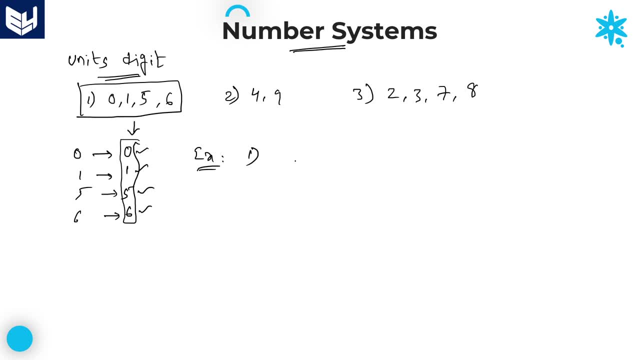 First question Here, the first example is: let us take 230 whole to the power of 125.. Here, as the number is looking very big number, As the number is looking very big number, Here we don't want This value. What is 230 power 125.. We don't want that value right. Here. we want the value in which, as we are calculating, only units place. 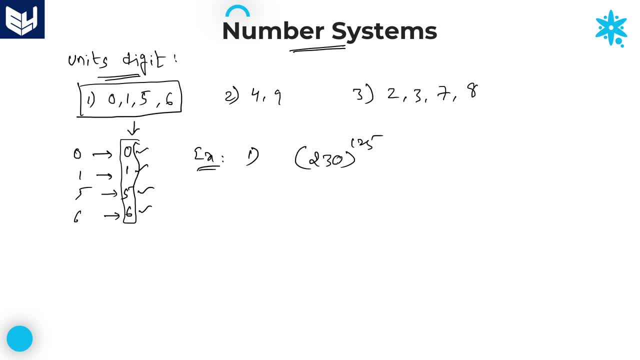 So I want only the units place digit of this number right Here in order to solve this one. First of all, you have to verify that. what is the number in which it is ending? Here the number is ending with 0.. Here the number is ending with 0.. That is the first point. 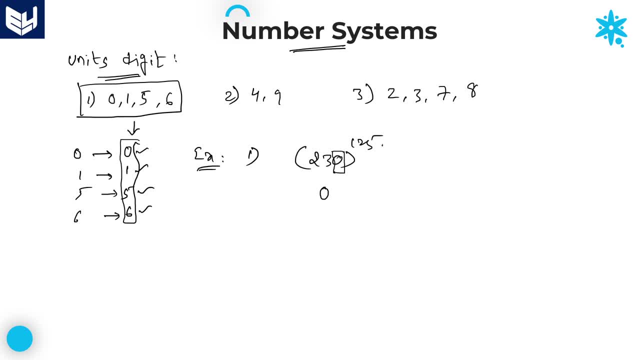 Whenever the number is ending with 0. And whatever the power value, Whatever the power value, Irrespective of the value of power, Then its units digit. Then its units digit is always the same digit. Then its units digit is always the same digit in which the number ends. 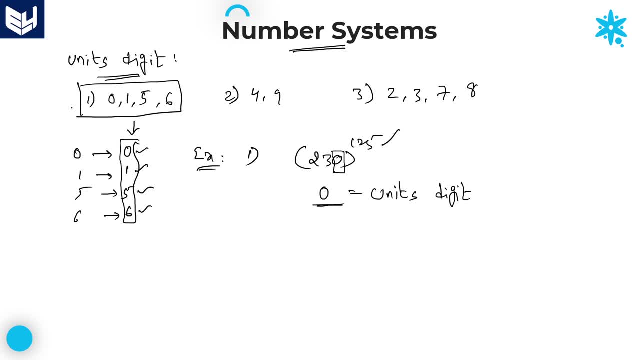 Here the number is ending with 0.. So it belongs To first category digits: 0, 1, 5, 6.. Right, So the required units place digit for this number is 0.. Suppose, for example, 125 whole to the power of 621. 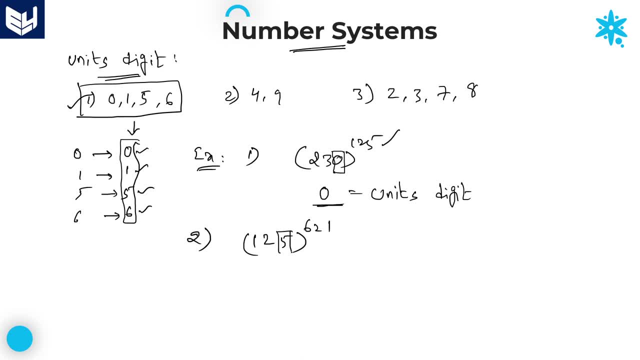 Here, if you observe carefully, The number is ending with 5.. The number is ending with 5. And whatever the power value, Irrespective of this power value, Then its units digit, Then its units digit is always the same digit in which the number ends. 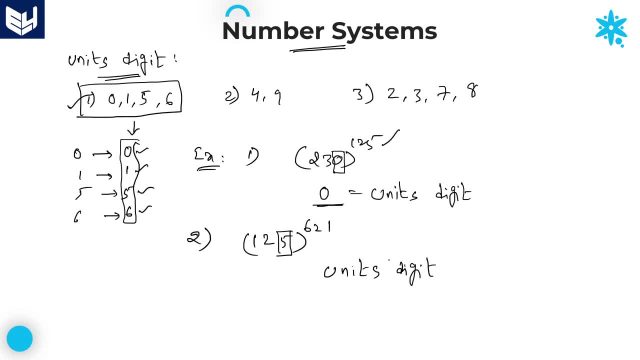 Here also, this number is belongs to first category digits. So the required units place digit of this particular number, 125 whole to the power of 621., Which is equal to 5.. That is the required answer for this question, Guys. first category digits. is very simple to get the answer. 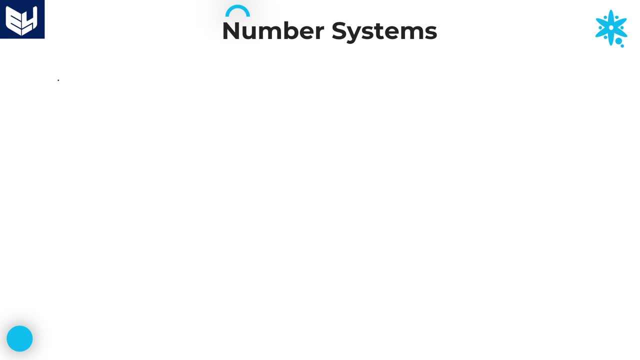 How to calculate units place digit. Let me explain one more. For example Here: 2136.. Whole to the power of 789.. 2136, whole to the power of 789.. What is the units place digit of this particular number? 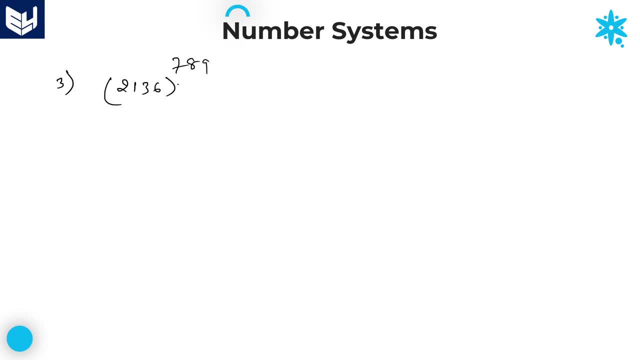 So many students are afraid of just by seeing the number itself. But if you know the concept Definitely, it is very simple task to get the answer Right, As we are calculating Only the units place digit. Here the number is ending with. 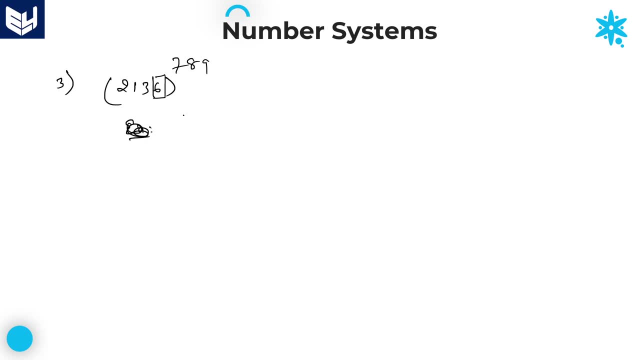 Just observe this number. Here the number is ending with 6.. So it belongs to first category digits. In first category digits what is the rule? Whatever the number is ending with That number itself is the units place digit. Therefore here also units digit is 6 only. 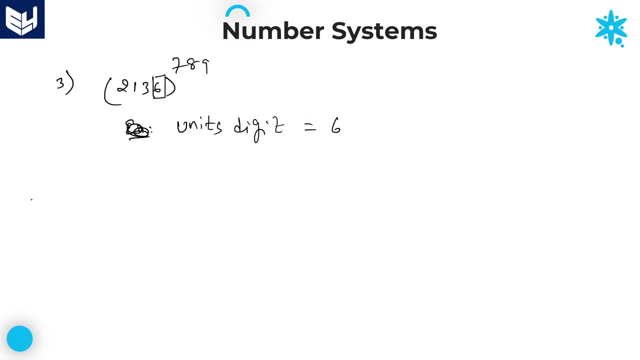 Here also units. digit is 6. only Now I will explain how to solve the problems whenever: addition of two numbers, Subtraction of two numbers or else multiplication of two numbers. I will explain those kind of things. Let us suppose that 215 whole to the power of 126, plus 621 whole to the power of 120. 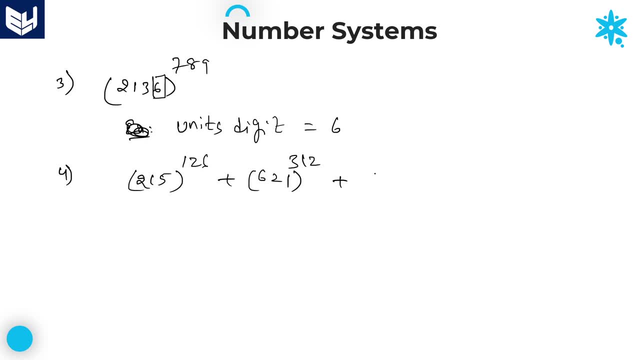 312 plus 526.. 526 whole to the power of 458.. This is a number. What is the units place of this number? What is the units place or units digit? Both are same. What is the units digit of this entire number? 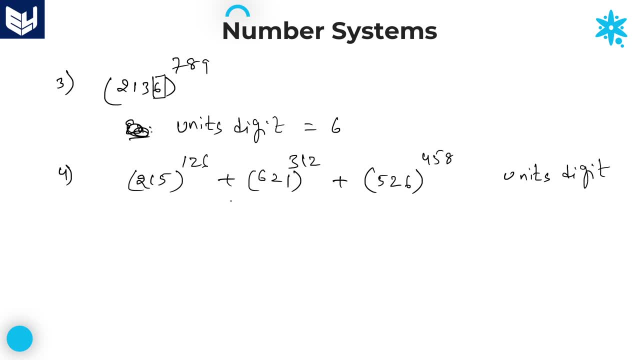 Here he is not asking about the individual, But he is asking about the individual values of units place, digit of each and every number. He is asking us to calculate what is after adding all these numbers. What should be the units place of that particular number? 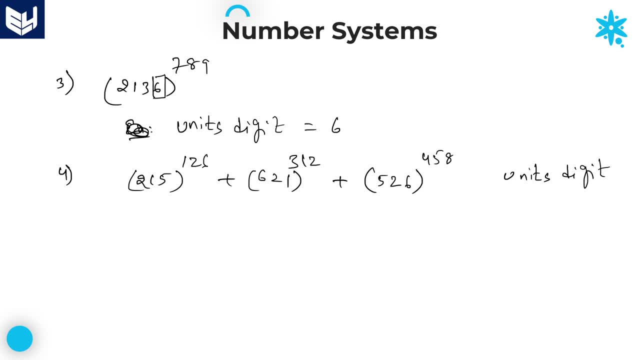 Whenever these kind of problems are asking, You just take individual values first. Here, if you observe carefully, the number is ending with 5.. Whatever the power value units place is always 5.. Here the number is ending with 1.. Number is ending with 1.. 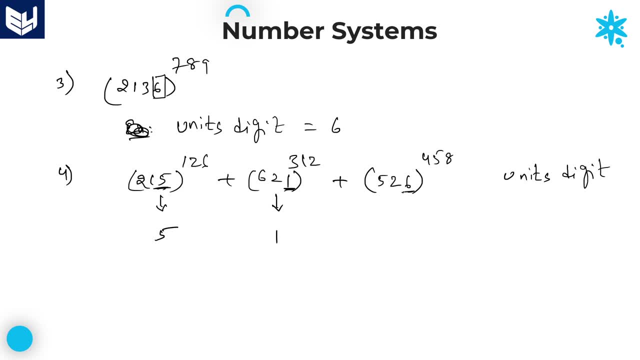 And whatever the power value units place is 1.. Here the number is ending with 6.. Whatever the power value units place is 6.. Now, after getting each and every individual units place digit, Then what you have to do is You need to add all the values. 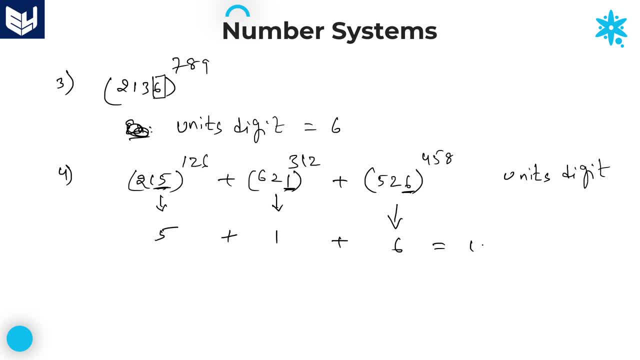 5 plus 1, 6. 6 plus 6, again 12.. 5 plus 1, 6.. 6 plus 6, 12.. Now, if you observe carefully, The units digit of entire all these numbers, which is equal to 2.. 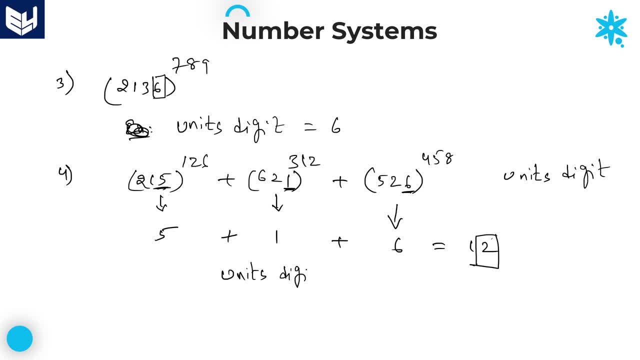 Units, digit of all the numbers which is equal to 2.. In this way we can solve the problems related to this model Whenever any arithmetical operation, not only addition, We can also do for subtraction and also multiplication, Most of the cases in examination point of view. 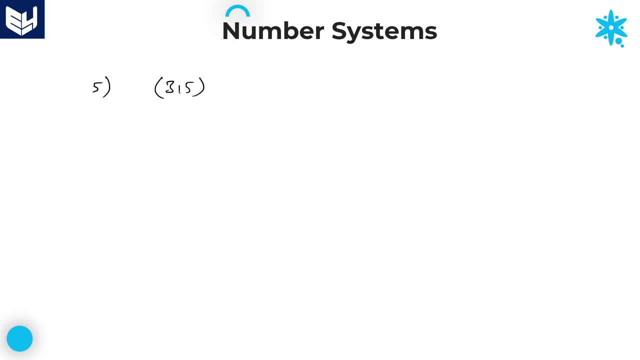 There is a chance of giving a multiplication. Multiplication is possible in examination point of view I am talking about. Let me take one more example here. This is multiplication, symbol Multiplication. It is very easy to identify that. what is answer? 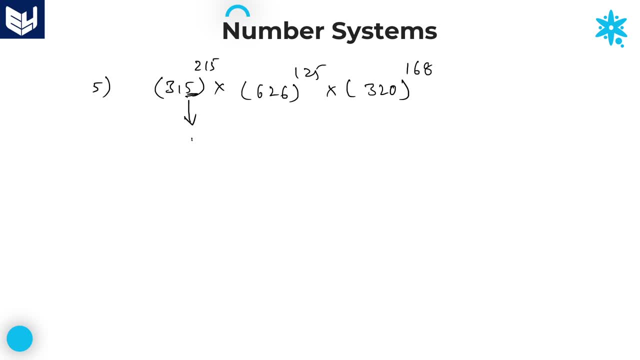 Here, individually, the number is ending with 5.. Units: place is 5.. Here the number is ending With 6. units- place is 6. here the number is ending with 0 units- place is 0.. Now you can multiply all the values: 5 into 6, 30, 30 into 0: 0. units: place of all these numbers: 0.